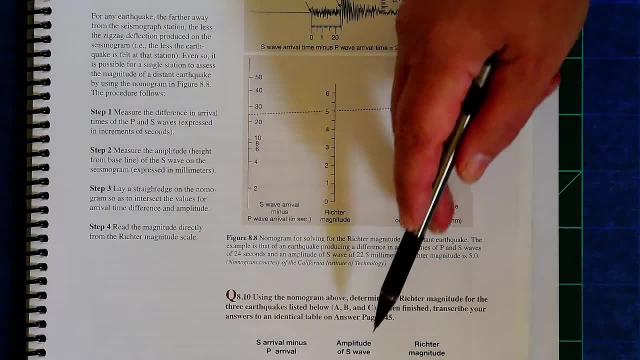 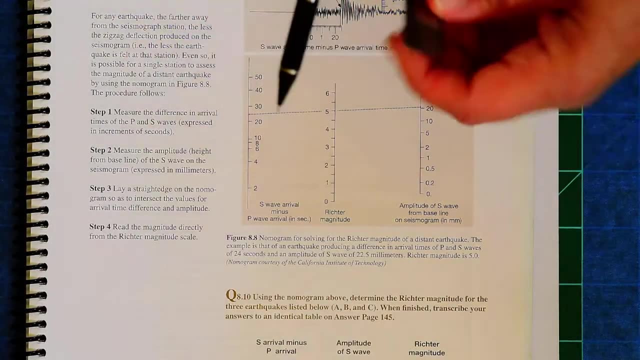 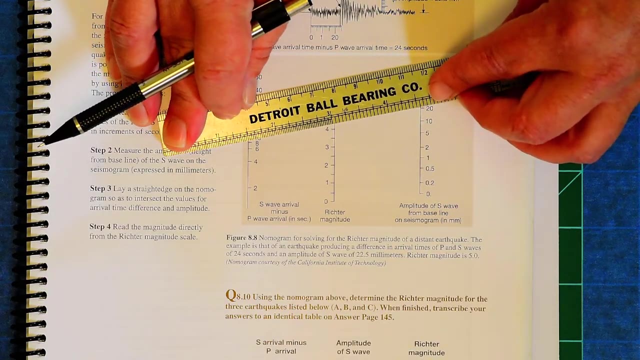 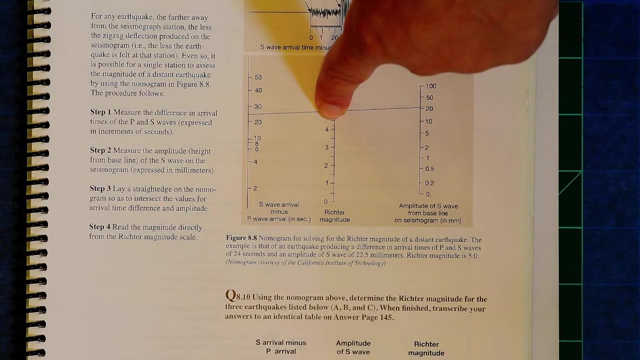 part of the graph and 8 would be right there. You have 20 millimeters of amplitude, which is right there. So you will take a straightedge line 8 up with 20 and wherever it crosses, that's what your Richter magnitude is. So just make. 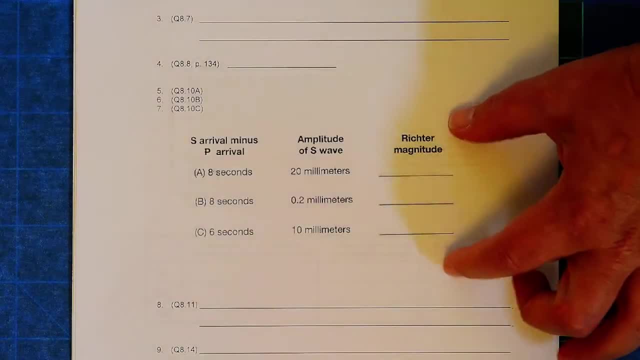 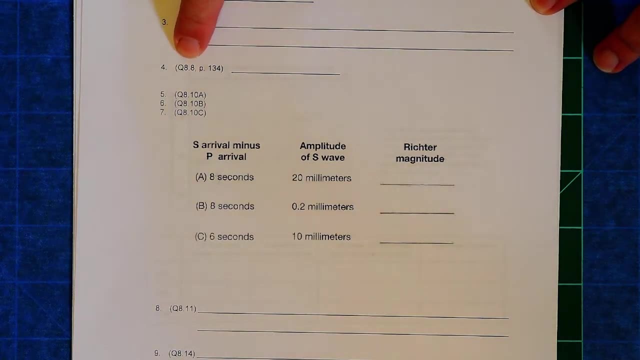 sure that you use this graph for these three questions. Oh, and I do need to point out something on this one: Your lab book has a typo and there are two question 8.8s. I want you to answer the one on page 134, so make sure you. 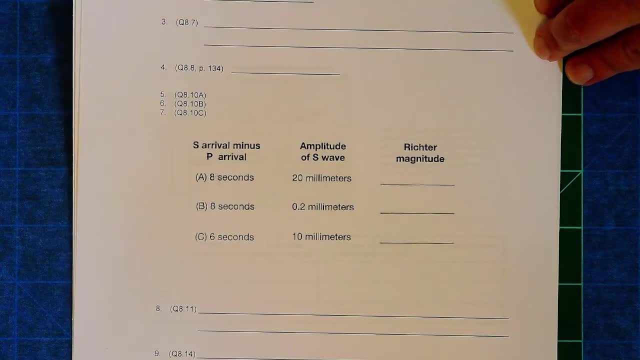 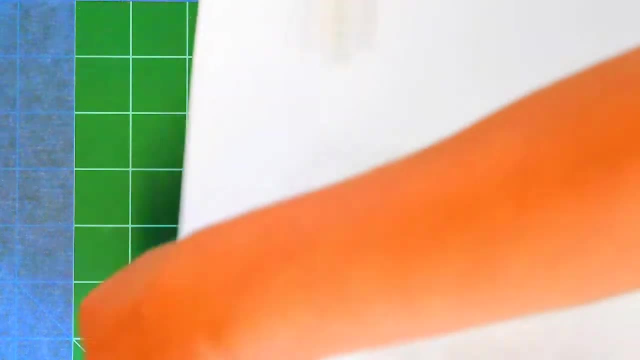 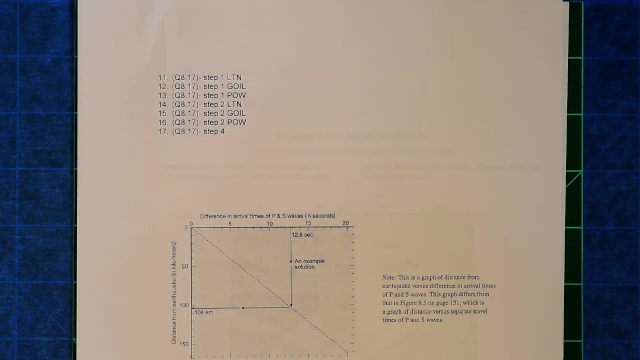 pay attention. Pay attention to that and don't answer the wrong question 8.8.. Okay, another part of this lab is these questions here. This is where you are going to actually figure out the epicenter of an earthquake, given real data. You're going. 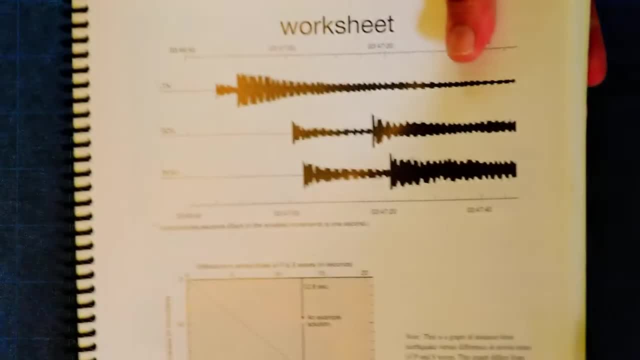 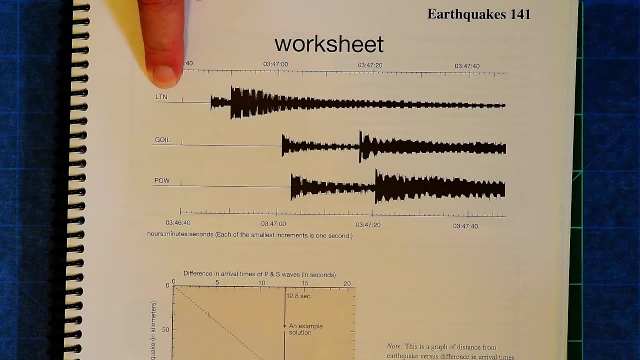 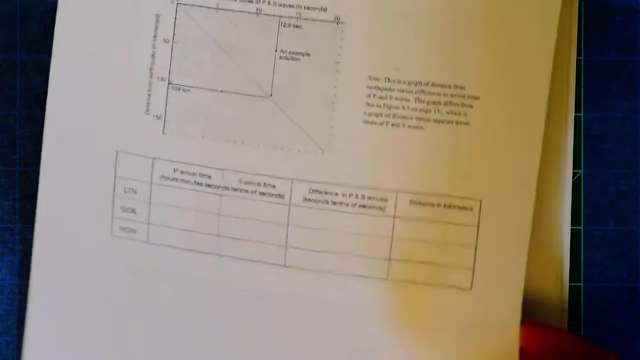 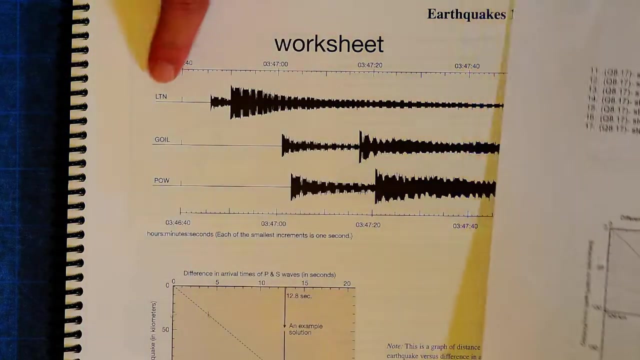 to be given real seismograms and those are shown right here We have the seismogram at station LTN, the one at GOIL and the one at POW, And on your lab you have this chart to fill in. So let's look first at LTN, Right? 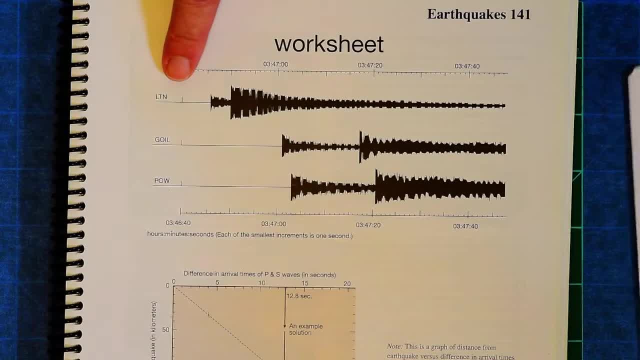 there we have LTN on the chart. So the first thing you want to measure is the P wave arrival time And remember that you want to measure the P wave arrival time. So remember, on these, the P wave is the first wave to arrive. The S wave is the second. 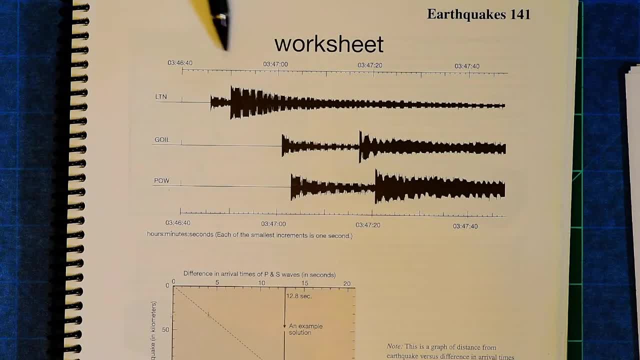 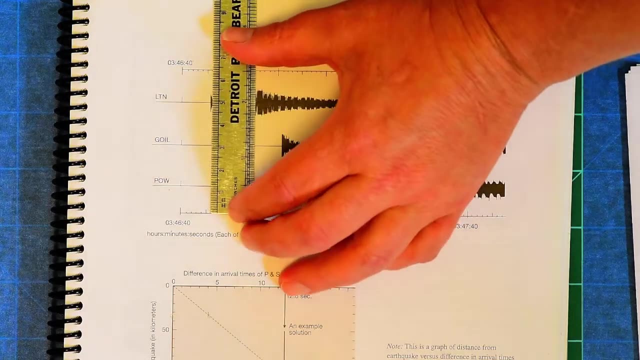 Time is going in this direction. Up here on this graph, we have time shown in hours, minutes and seconds. So right here is where the P wave first arrives, And so I'm just going to put my ruler there and say: alright, the P wave first arrives, So let's set a. 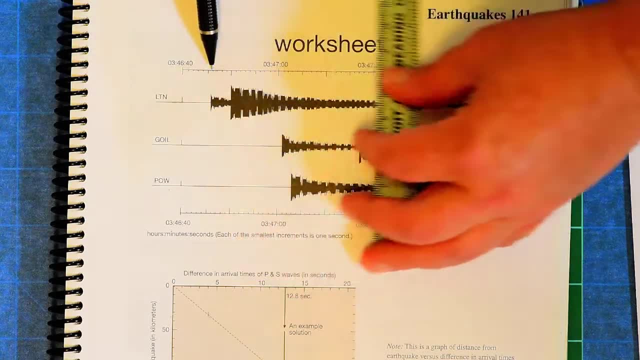 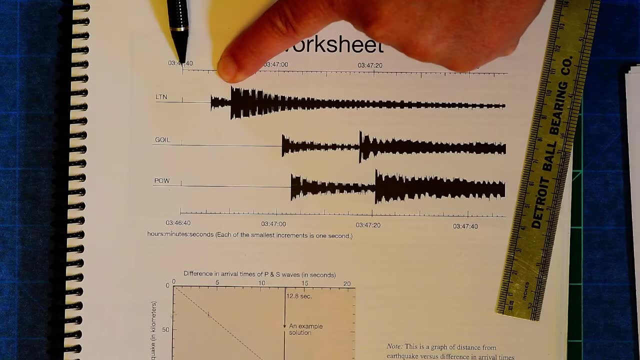 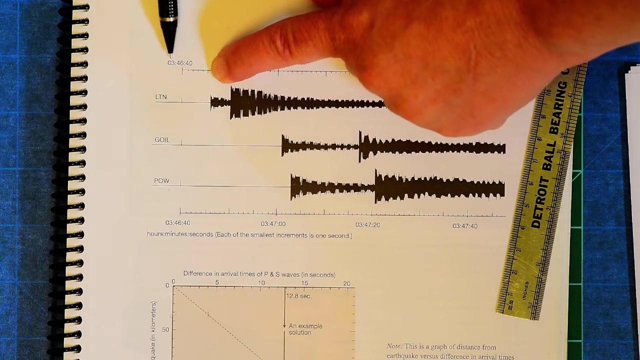 P wave First arrives right here, right at that little thing. so this is 3 hours 46 minutes 40 seconds. that's 3 hours 47 minutes 0 seconds. that's 40 seconds. 50, no 40, 45, 50, 55. there's the next minute, and if our P wave arrives right there, that means it's. 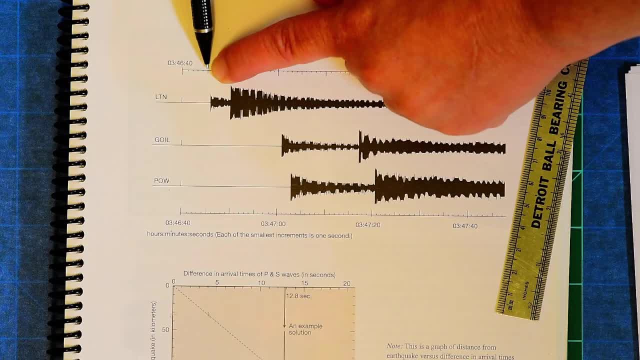 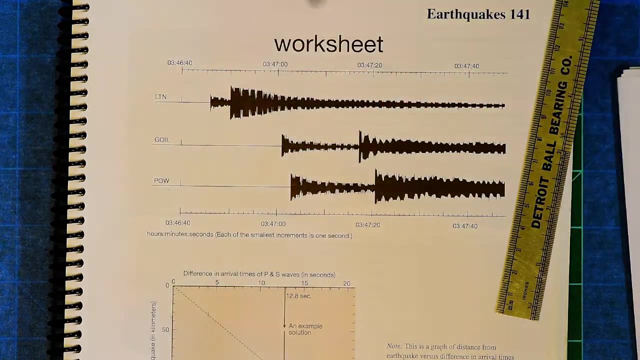 3 hours 46 seconds. I just said that wrong, sorry. 3 hours 46 minutes, 45 seconds. right, because there's. this is 40, 41, 42, 43, 44, 45, and so that is what you would write up down here. you would write 3 hours. 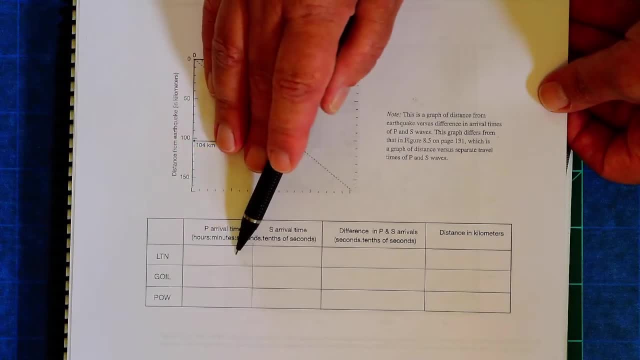 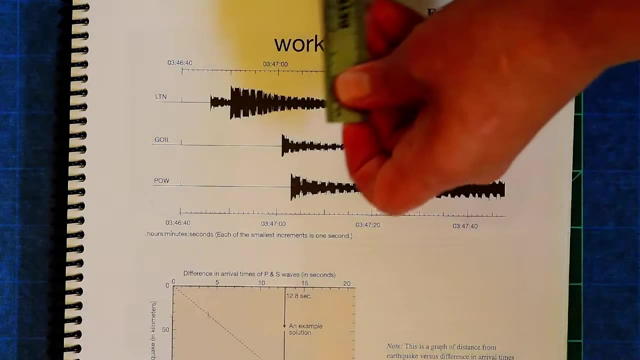 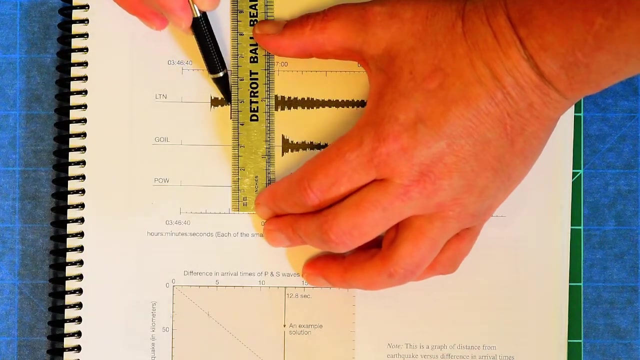 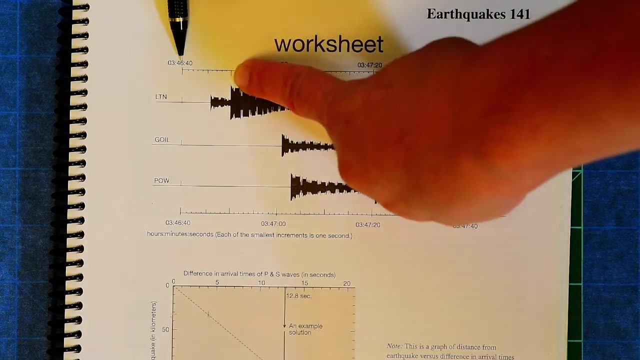 46 minutes 45 seconds. then the next thing you do is figure out when the S wave arrived. so again, I'm just gonna set my ruler right here. looks like the S wave arrives right there. well, guess what? that's 3 hours 46 minutes 50 seconds. 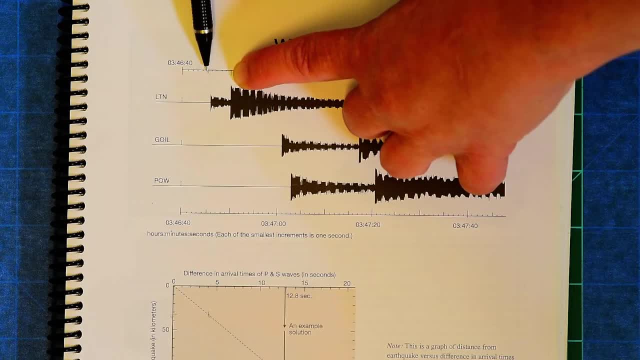 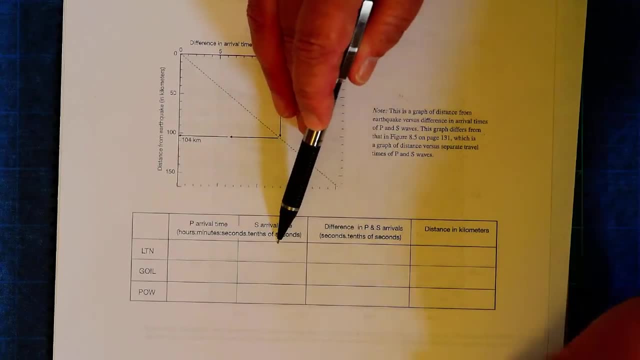 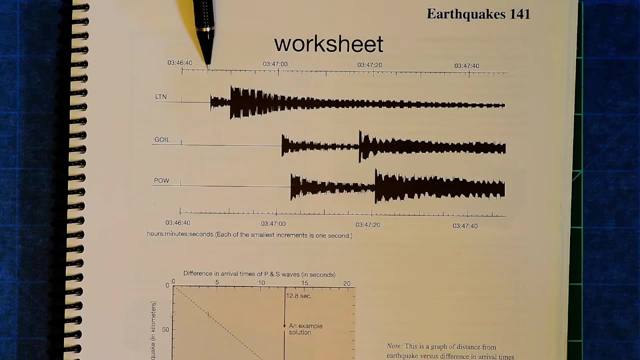 right, each one of these little marks is a second. that's 5, 10, that's 3, 46, 50. so I would write that right here now: the difference between the P and the S waves. if one arrived at 45 seconds and one arrived at 50 seconds, the time difference. 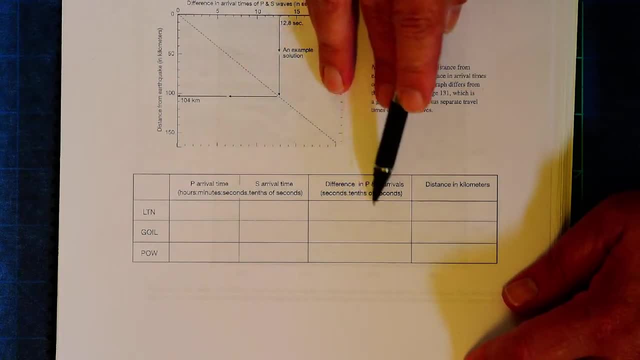 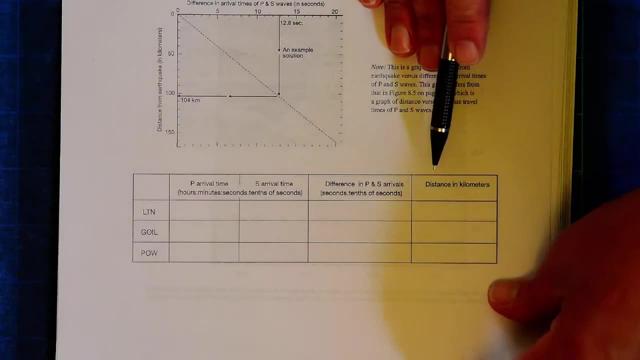 would be 5 seconds, which is what you write in here. and now that you have the difference in the P and the S, the time difference between the P and the S is 50. now the difference between the P and the S is 50. the s-wave arrival times. we can calculate the distance in kilometers And this distance in. 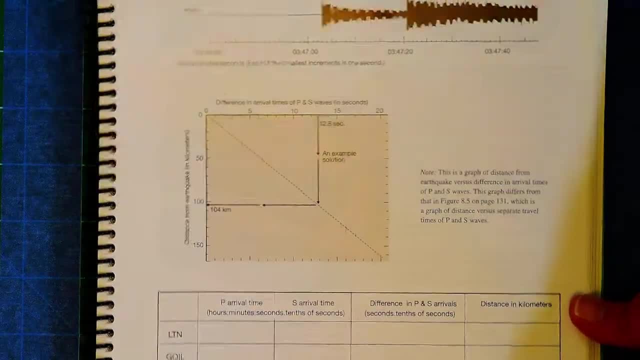 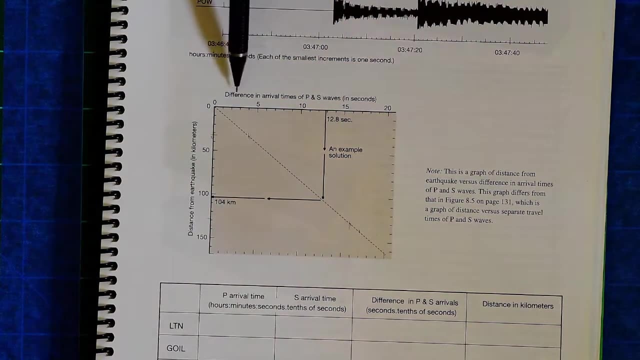 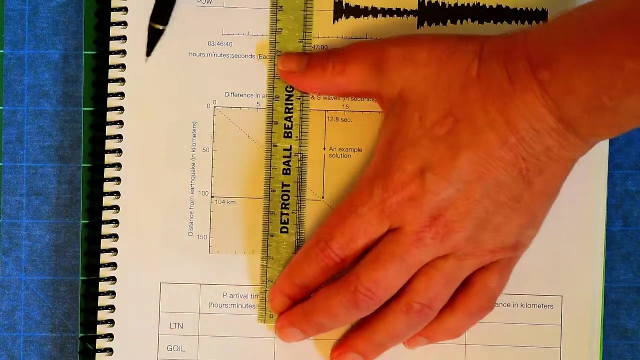 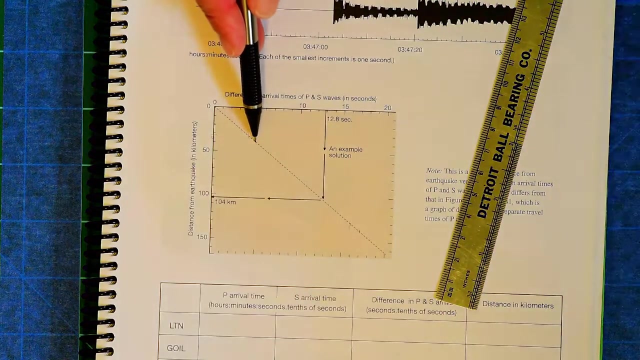 kilometers. we can get off this chart right here. So on the x-axis we have the difference in arrival times of the p and the s-waves. Right, there is five seconds. right, We said it was five seconds, So there's five seconds. I go straight down from five seconds to this dashed. 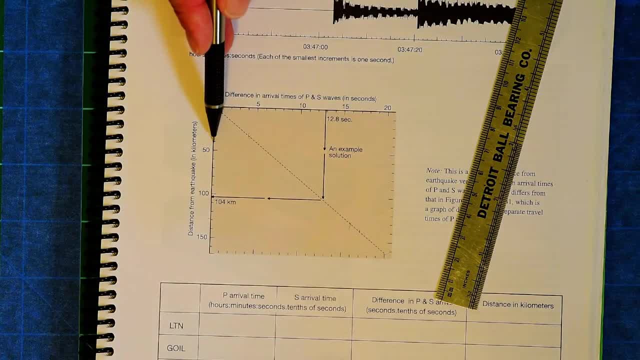 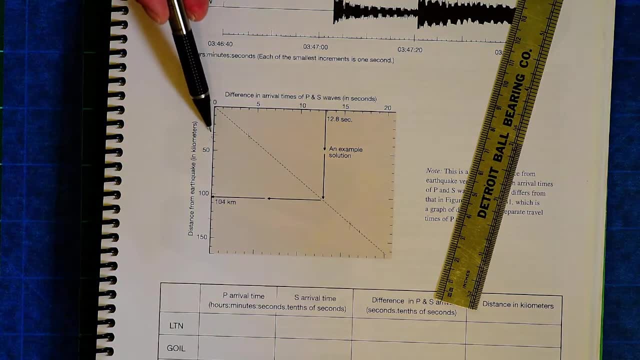 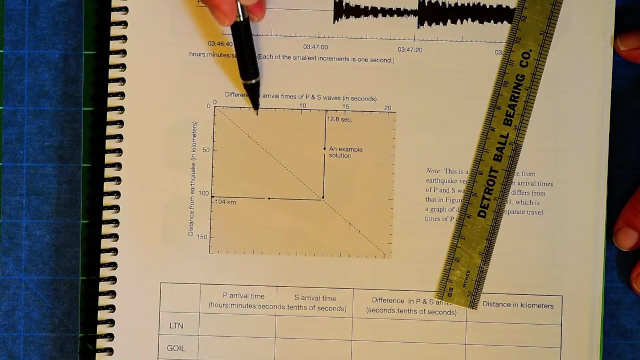 line and then I come straight across and that gives me the distance from the earthquake in kilometers. So that's five, ten, fifteen, twenty. no, this is ten, twenty, thirty, forty. Each one of these marks is ten. So if I came down here and straight across, it looks like I'm sitting right. 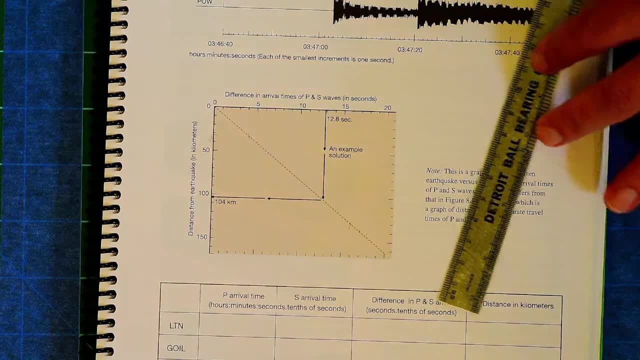 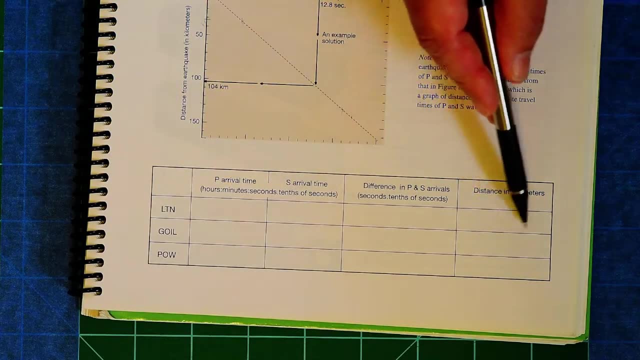 at the p and the s-wave, So that's five seconds. So that's five seconds. So that's five seconds At forty kilometers. So that's what you're going to do with those problems. We just figured out the one for LTN and we know that's forty kilometers away from the epicenter of the. 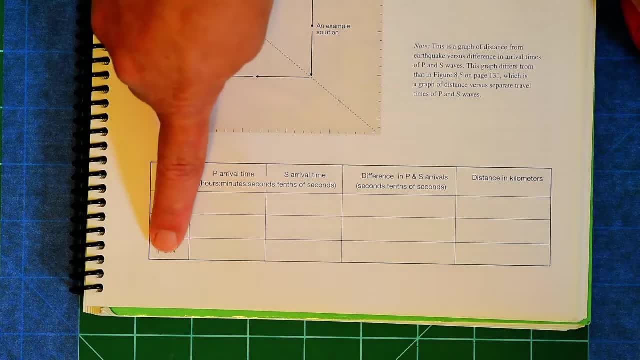 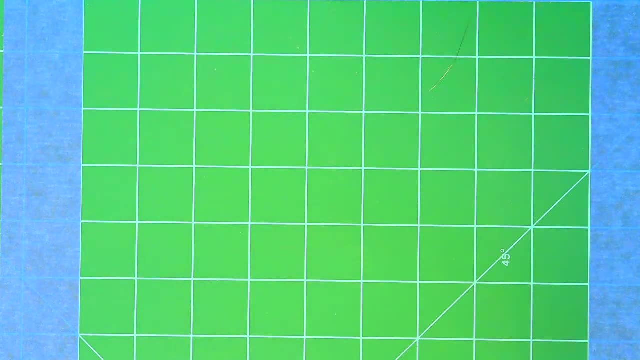 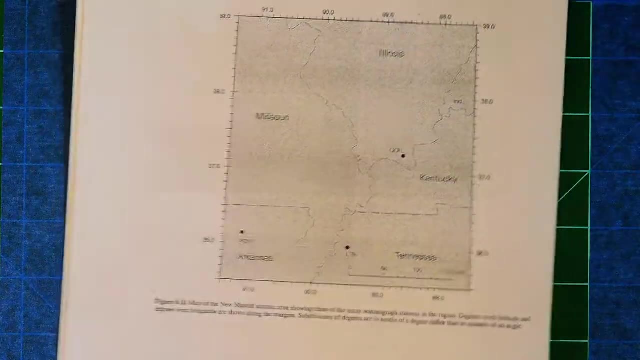 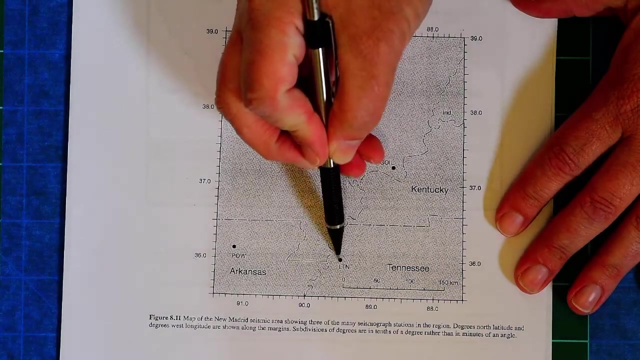 earthquake. You now need to fill in the ones for the other two seismograms. All right. Additional problems that you will have with this include, um, then locating the epicenter of that earthquake. You have this, and remember, we just calculated. 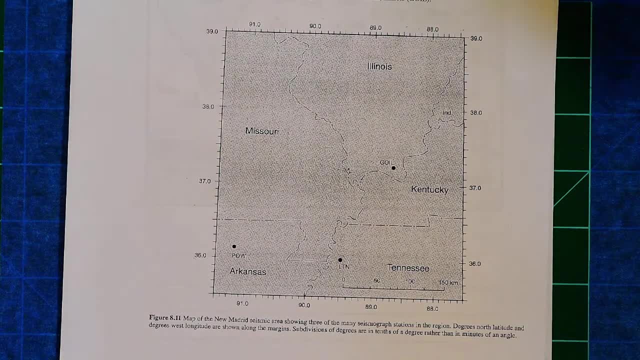 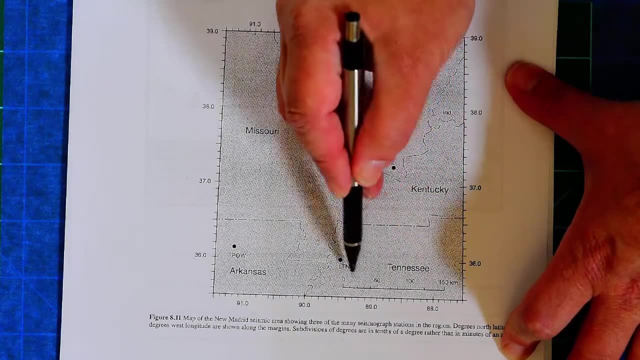 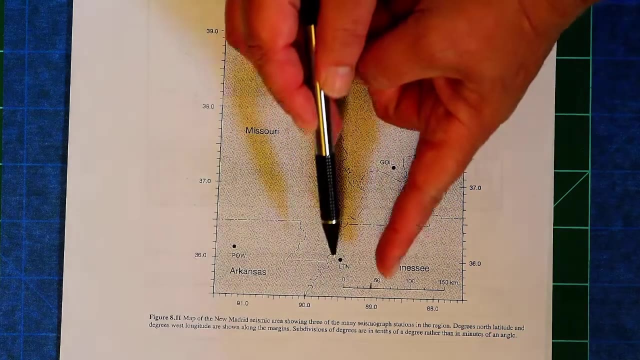 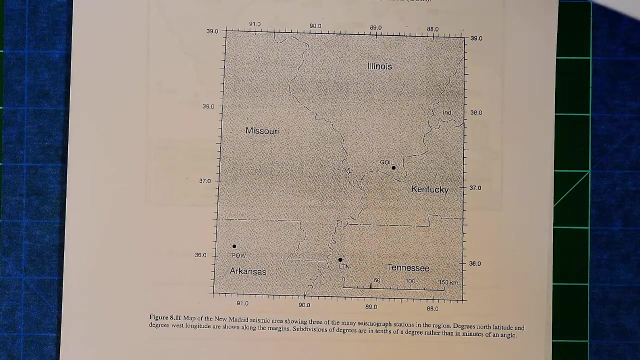 LTNs um the distance to the earthquake from that. Well, here's a scale and we figured out it was forty kilometers away. Now if you happen to have a compass, you'll just set the compass to do forty kilometers and draw a circle. I know some of you don't have compasses at home, so you can. 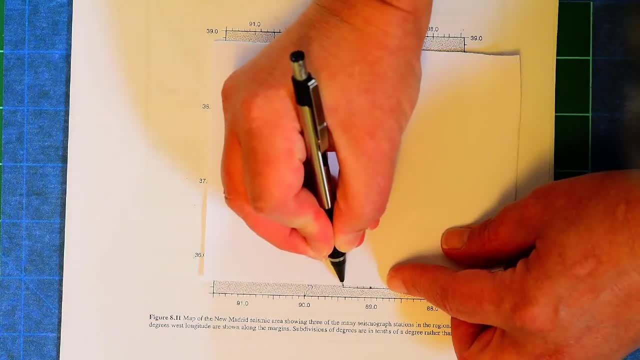 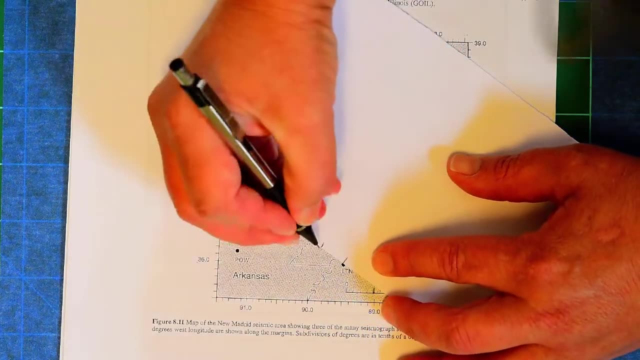 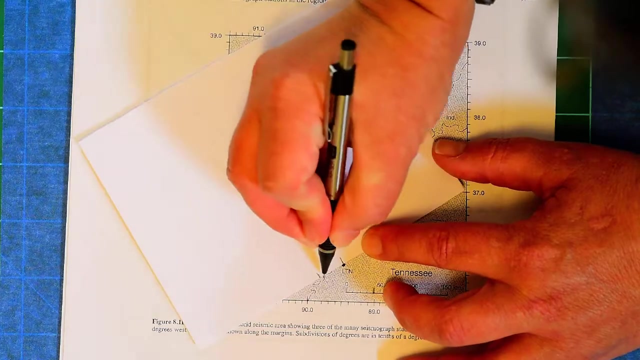 just take a piece of scrap paper and you can say, all right, there's zero, there's forty kilometers, there's LTN, and you can estimate what a circle would look like by putting a few marks along here. It's kind of like, uh, having a homemade compass. 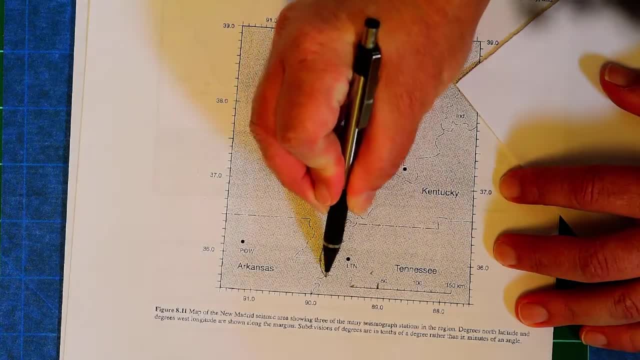 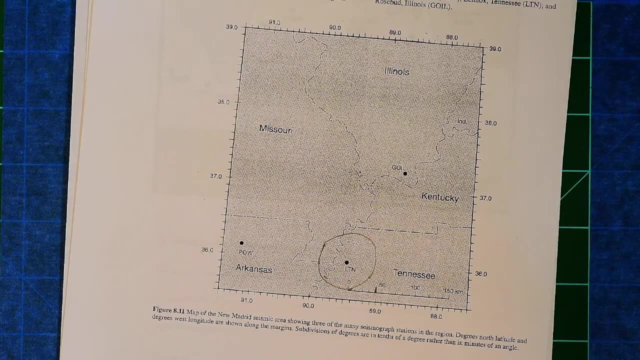 and from that you'll be able to estimate where your circle would be. I don't expect you to be perfect on these, but eventually, when you figure out the distances for these other two seismometers, you'll figure out approximately where the epicenter of the earthquake is, and you don't have to give me the 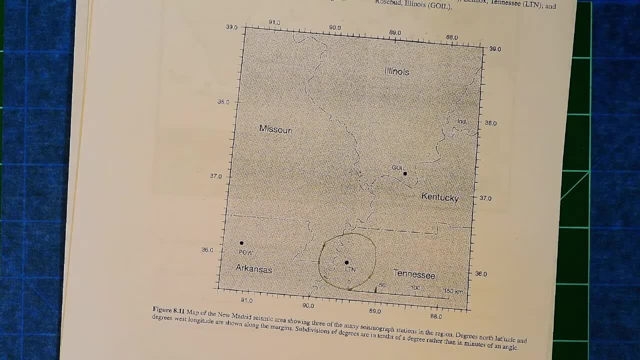 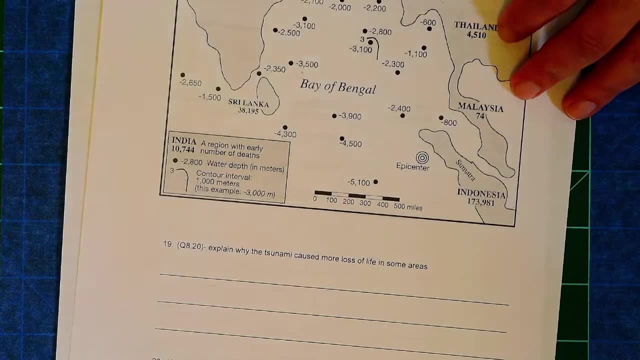 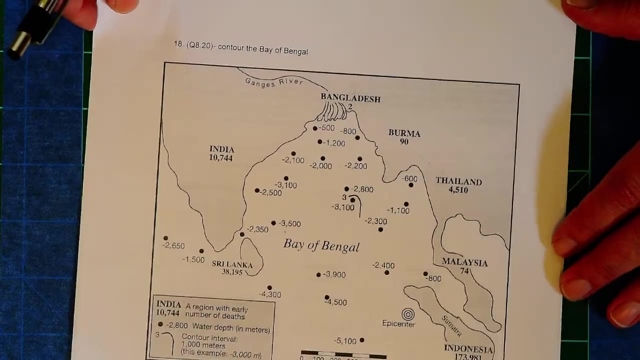 latitude and longitude or anything like that. just tell me approximately where it would be located. just come up with that in words. Alright, now last of the- well, second to last of the somewhat challenging questions that we have is here question number 18, where it says: 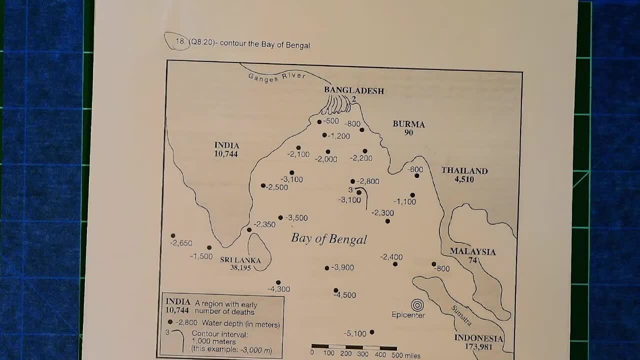 contour the Bay of Bengal. alright, I understand many of you have not had physical geology, so you don't know how to contour things. that's why we're going to do this problem together right now. when we contour things, what we're doing is we're either showing the 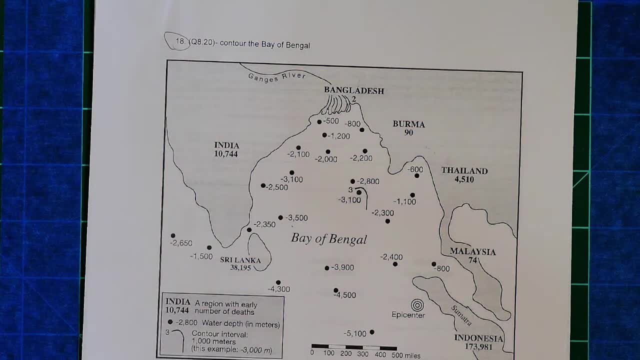 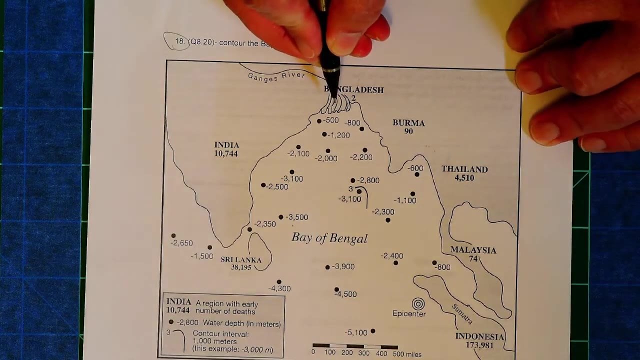 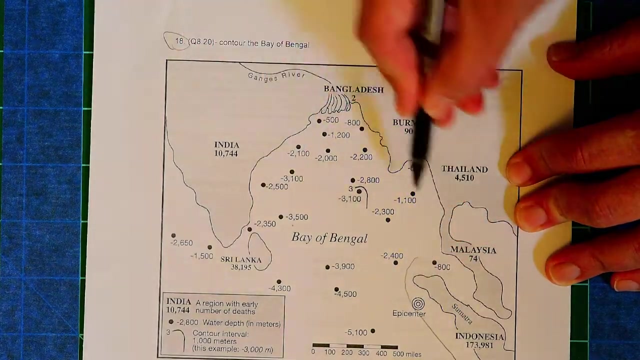 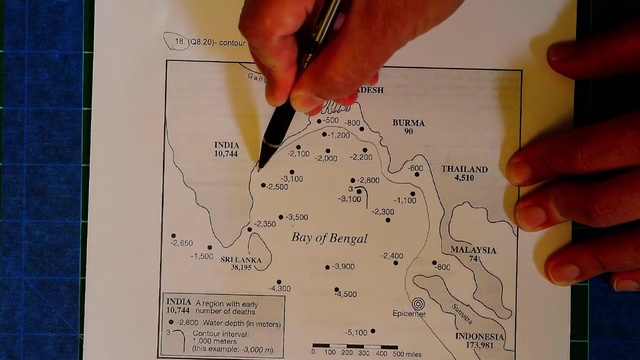 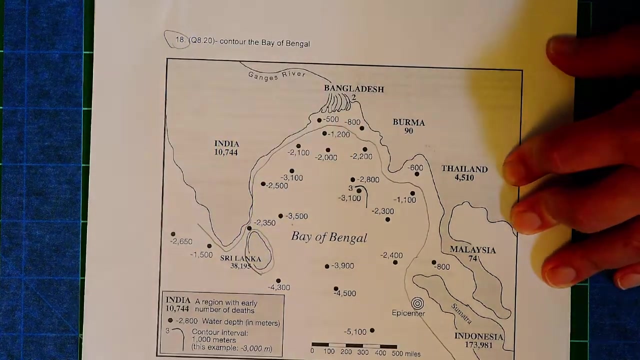 elevation above sea level or the depth below sea level. in this case, we're going to draw in the depth below sea level in thousands of meters. so, for example, let's see, let's draw in a thousand meters and draw that in, right about here. this is an island, so there's a thousand meters, right there. 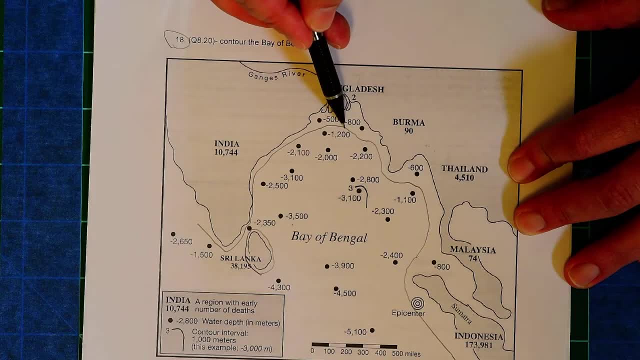 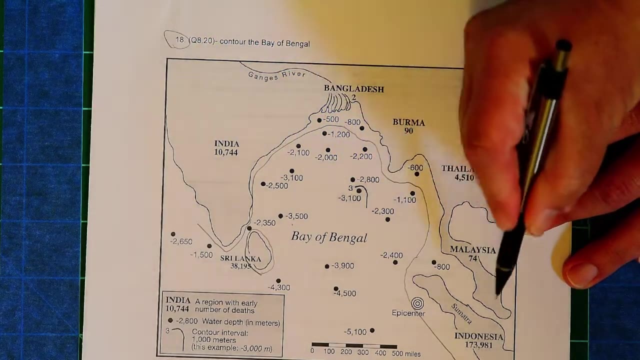 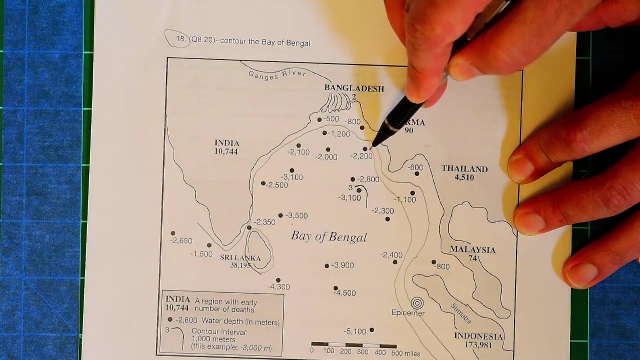 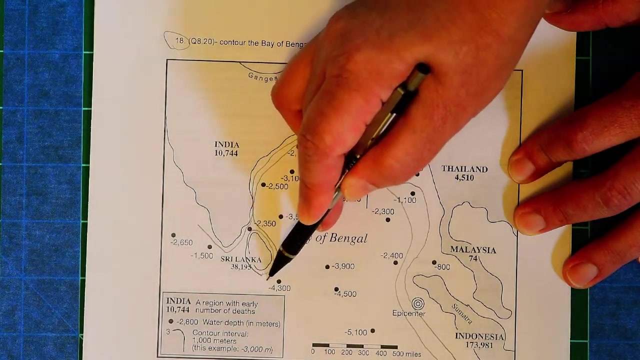 now, why did I draw the line there? this is a thousand meters below sea level. everything on one side of the line should be less than a thousand meters and everything on the other side of the line should be more than a thousand meters. see that? now let's draw in 2000 meters below sea level. 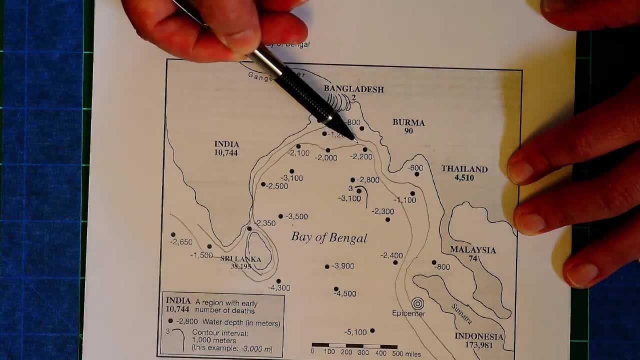 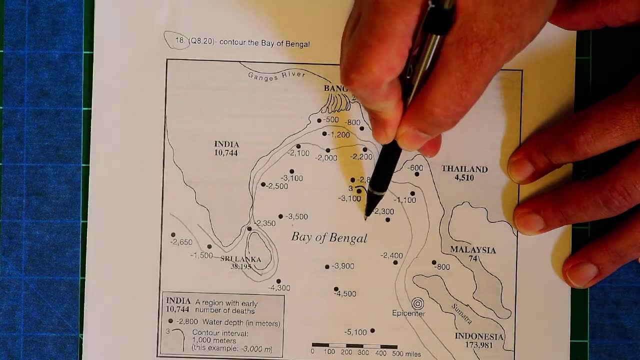 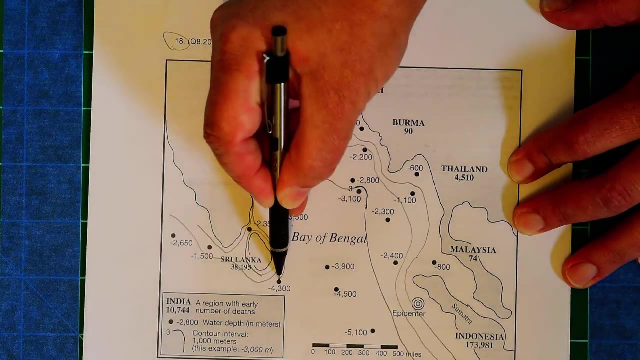 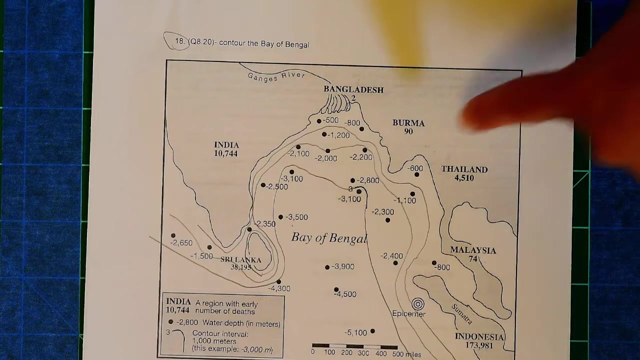 something like that. right again, everything on one side of the line is greater than 2000, everything on the other side is less. Then let's draw in 3,000 meters, and that should be enough to solve the problem. So hey, you get at least one point for free by having that right. 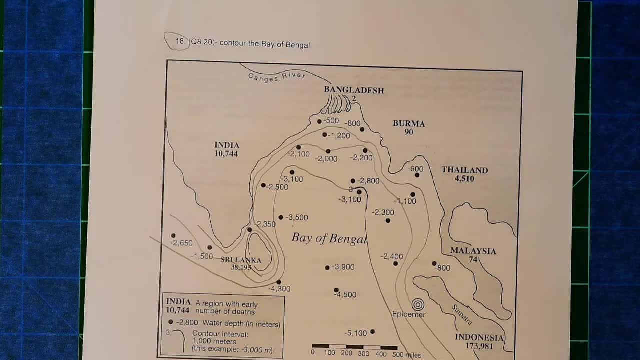 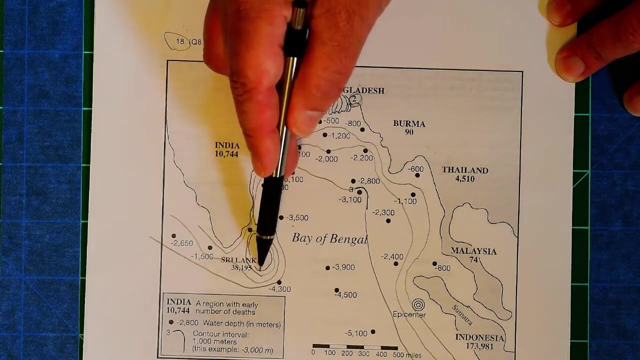 We did it together and one thing I want you to pay careful attention to, the reason you did this in number 18 is number 19 is going to ask you why, when there was a tsunami, only two people died in Bangladesh, but 38,000 died in Sri Lanka.